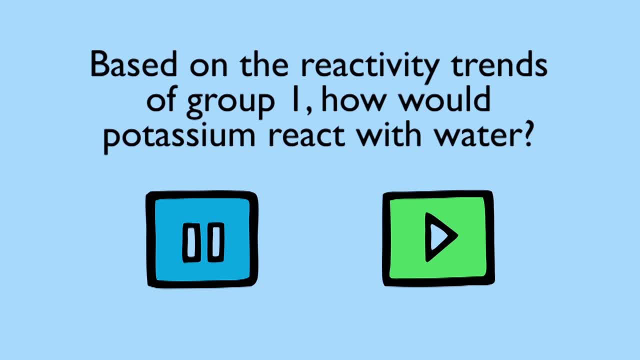 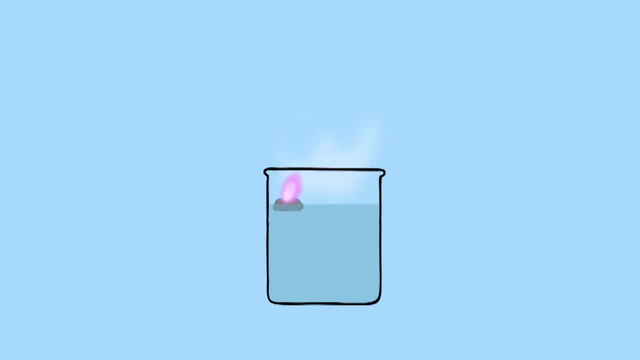 Pause the video and consider, then resume. Well, the chemical equation looks nearly the same, but the reaction is much more violent, because potassium is more reactive and enough heat is given out to ignite the hydrogen gas, and this then ignites the metal itself. 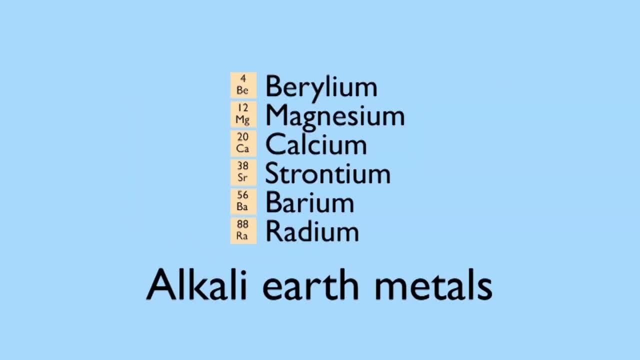 Moving on to group 2, the alkali earth metals, things are a little different. The metal at the top of the group, beryllium, is too inert to react with water. Magnesium just below it reacts only very slightly. 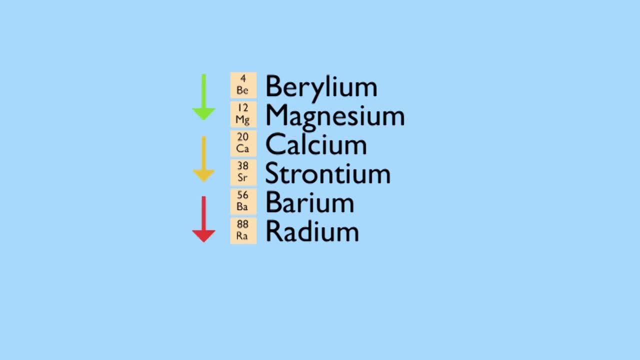 But again, consider the reactivity trend. It increases going down the group. The elements below calcium, strontium and barium will react with water to form their hydroxides, though in each case less vigorously. If we drop some strontium metal into our beaker of water, it will sink to the bottom. 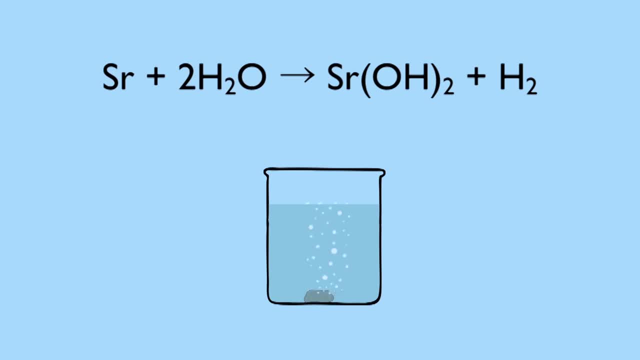 Small bubbles of hydrogen gas then appear on its surface, showing the reaction is taking place. You might observe a white precipitate, which is solid strontium hydroxide. Unlike group 1, the hydroxides formed by group 2 are only partially water soluble. 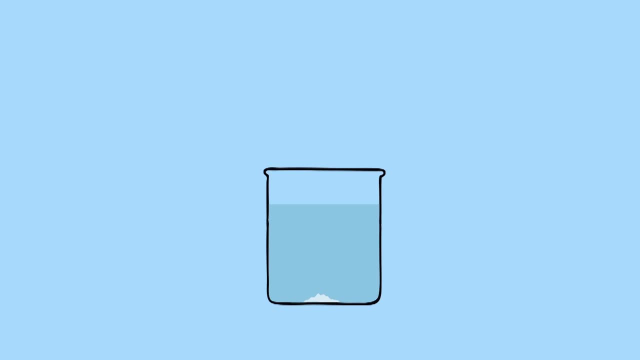 and can often be seen in the solid form as the reaction occurs. The solid hydroxide often forms as a protective layer on the surface of the metal itself and slows down the reaction. But the solution will still be basic, as at least a few free OH- ions are present. 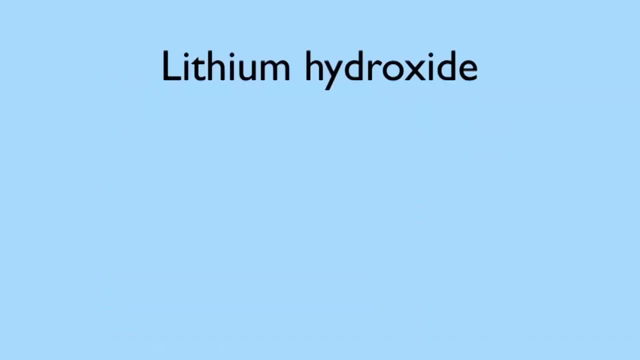 Metal hydroxides have many uses in industry. Lithium Hydroxide is used to make a highly water repellent grease. Strontium hydroxide plays a role in the manufacture of table sugar from the sugar beet crop, But you'll never see hydroxide in the soil. 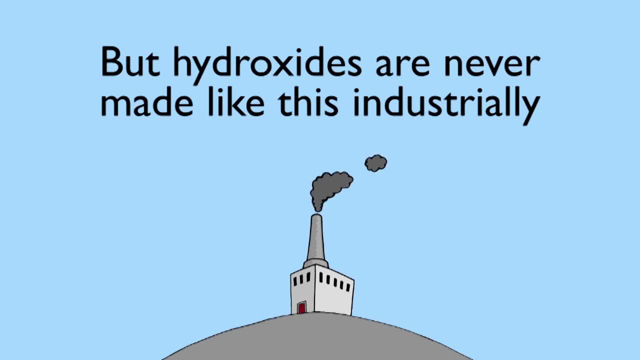 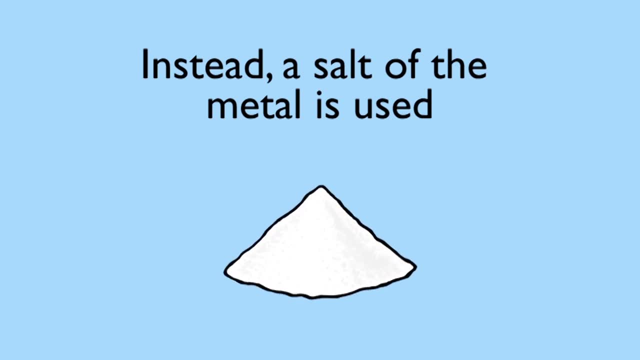 made in industry by adding the pure metal to water. It is far better to start with a salt of the metal, which is easier to make and cheaper to acquire. For example, strontium hydroxide is made by starting with the salt, strontium nitrate.